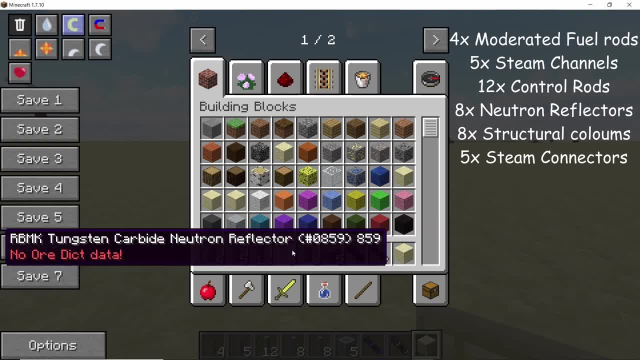 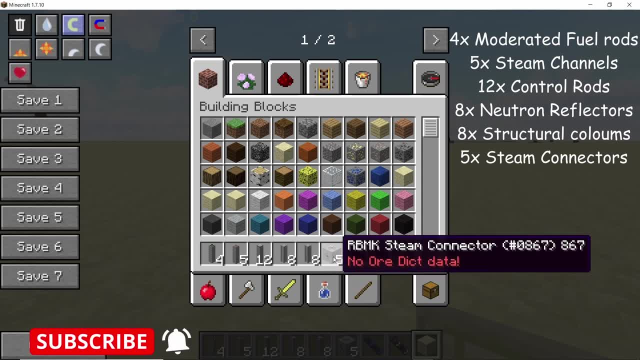 5 steam channels, 12 control rods, 8 tungsten carbide neutron reflectors and also 8 structural columns. Now you will also need 5 steam connectors and any temporary block. So take your temporary block and come 3 up from the ground. And on the third one, 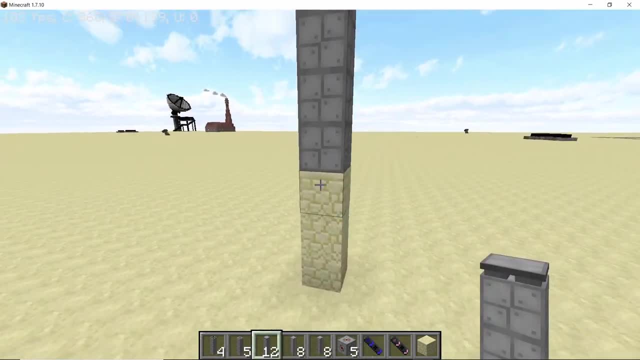 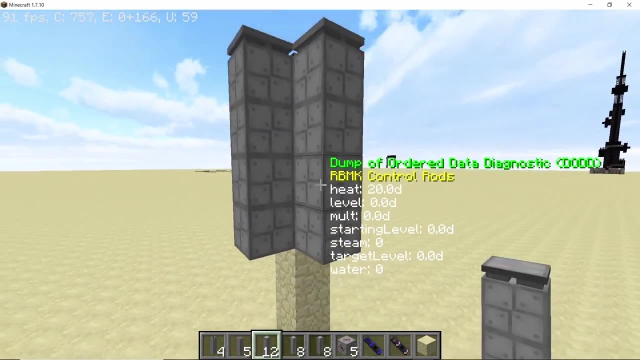 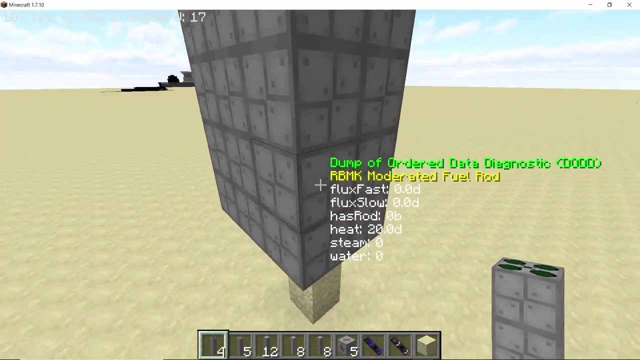 place down a steam channel. Now surrounding the steam channel, place down 4 control rods, 3 and the fourth one Now in the corners that you have just created. place down 4 fuel rods And make sure that these are the moderated fuel rods and not the normal ones. Otherwise, 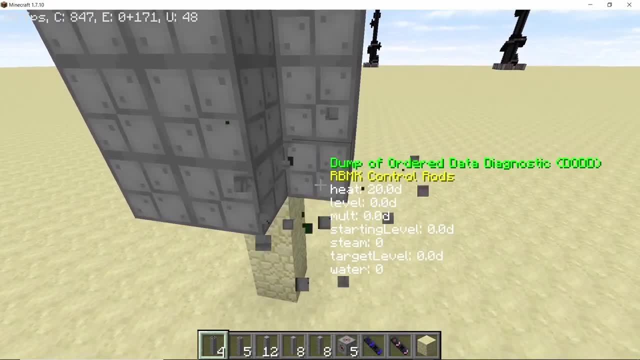 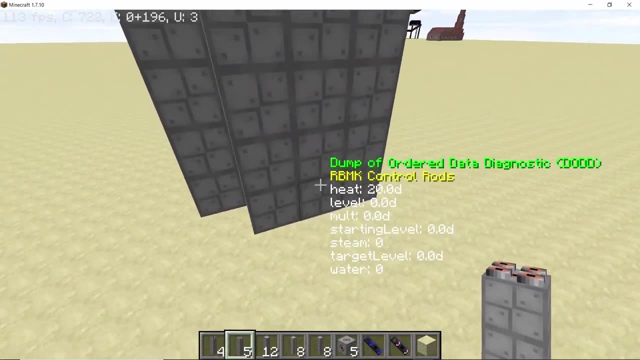 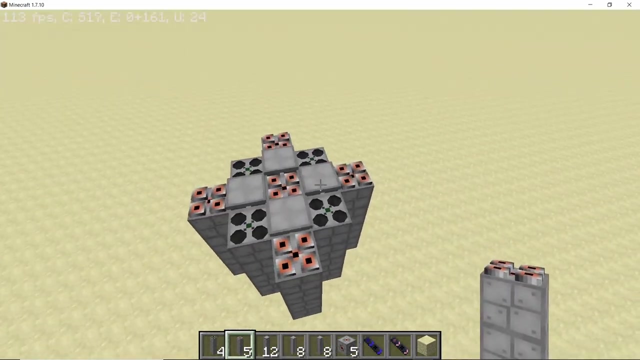 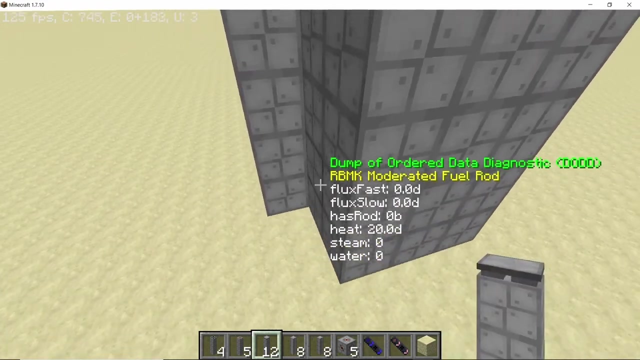 your reactor won't work properly. and the fourth one: it's now time to place down some more steam channels, so place one on each side, like this: three and four. now, beside each steam channel that we just placed, place down two control rods, one and two, and now do that on all the four sides. 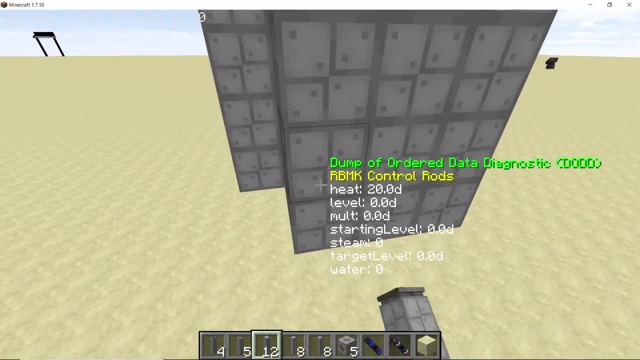 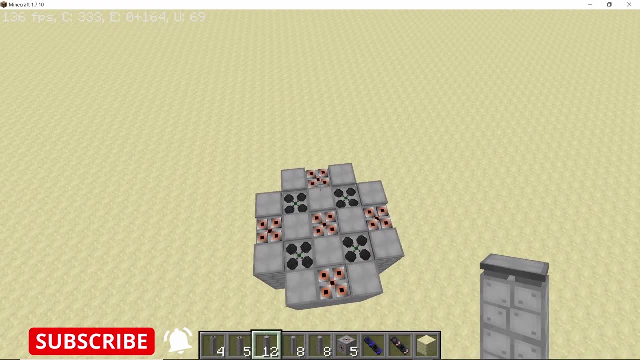 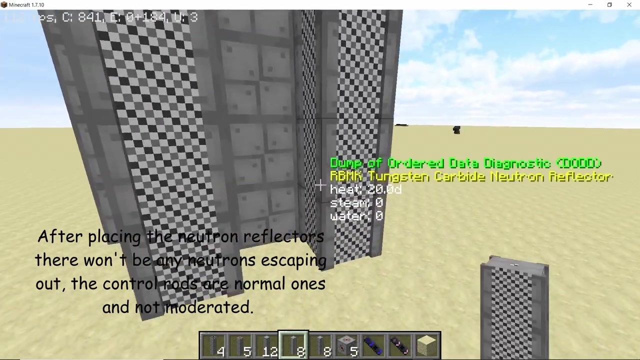 one, two, one and two and finally this last side. there we go, one and two, there we go. now it's time to place the neutron reflectors so that our reaction can be completed. so place down two neutron reflectors in front of the control rods that you just placed, two, and do that on all the 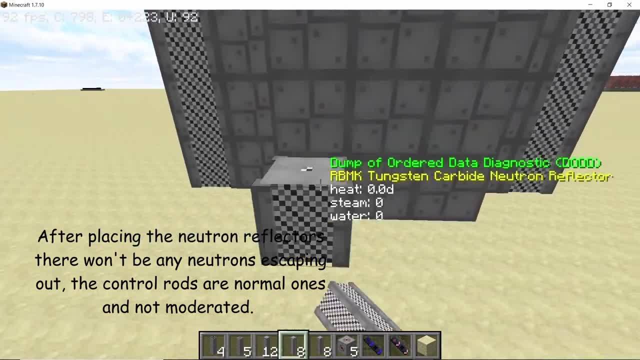 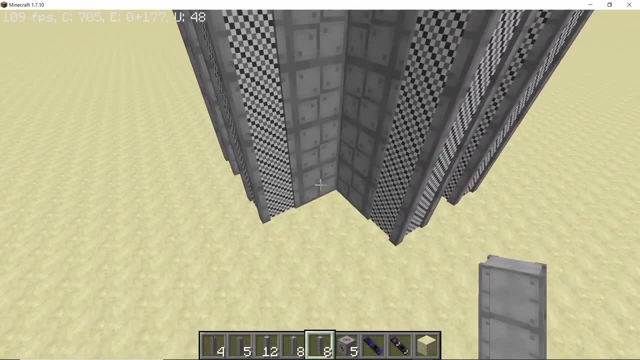 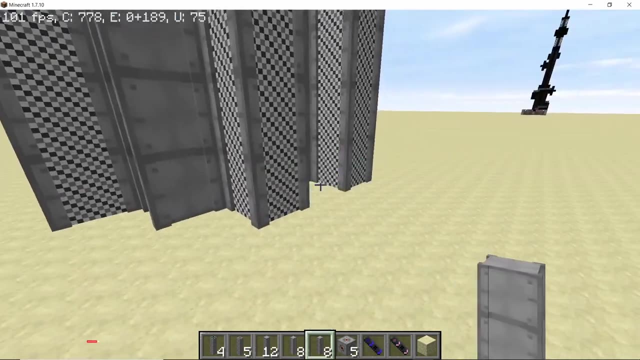 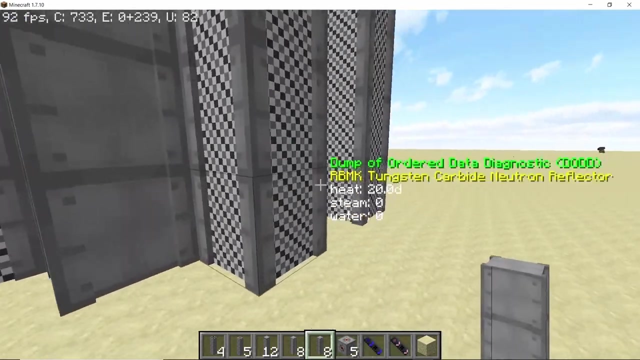 four sides. and here we go now. in all the remaining spaces, the corners that we have created, place down structural columns. you will need a total of eight: one, two, three, four, five, six, seven and finally the eight one, and with that the design of the rbmk is complete. 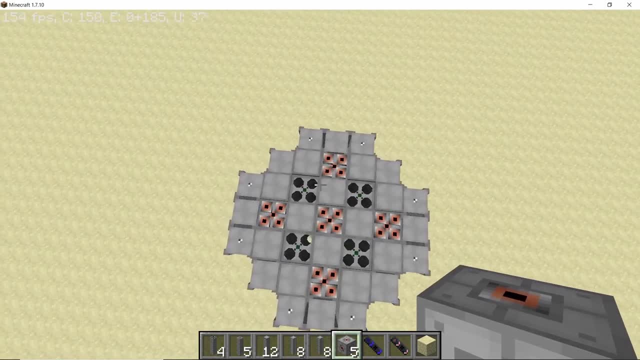 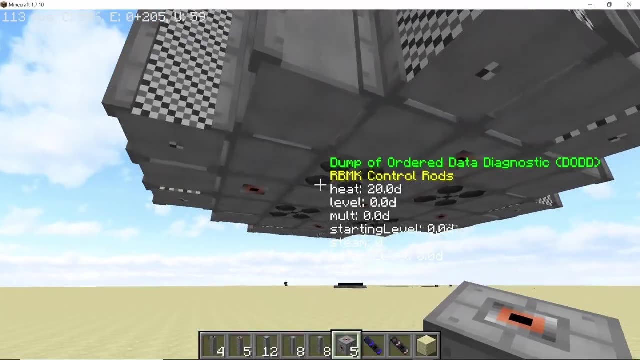 let's go over it one more time: five steam channels, four fuel rods and twelve control tubes, along with eight neutron reflectors. so this is how your rbmk should look like. now it's time for some piping, so connect some water ducts from the steam channels. 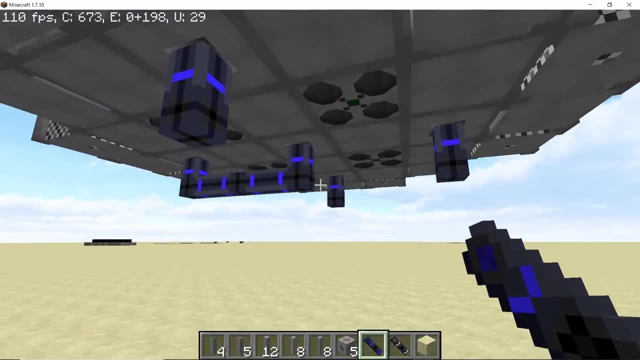 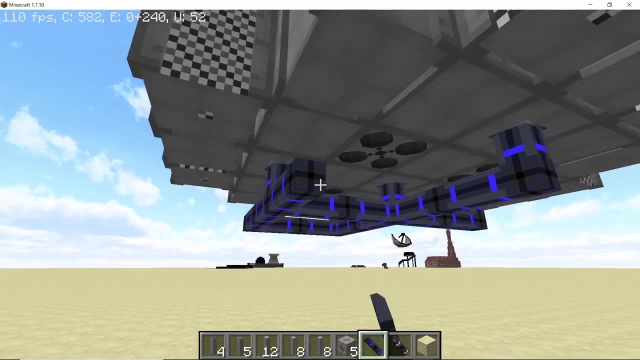 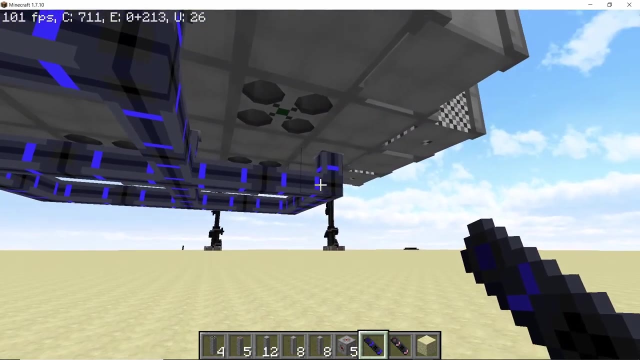 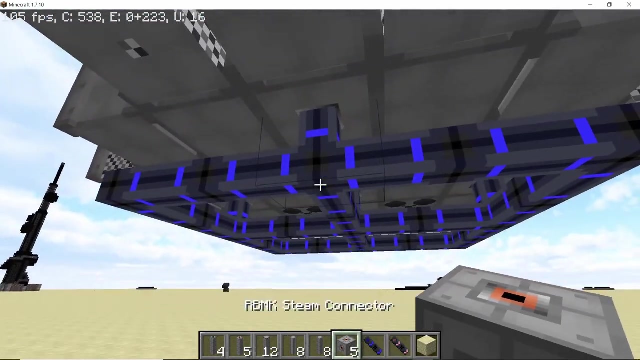 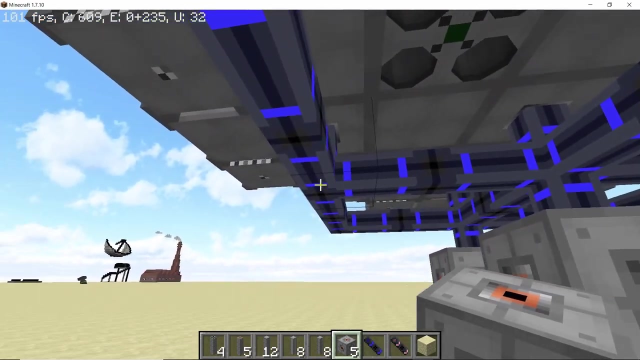 that you have placed and also connect them internally, like this, going to out, and do that on all the sides. and here goes the last one. now, beneath each of the steam channels that we have placed, let's place down our steam connectors. so we'll need a total of five steam connectors and the last one and from down the steam connectors. 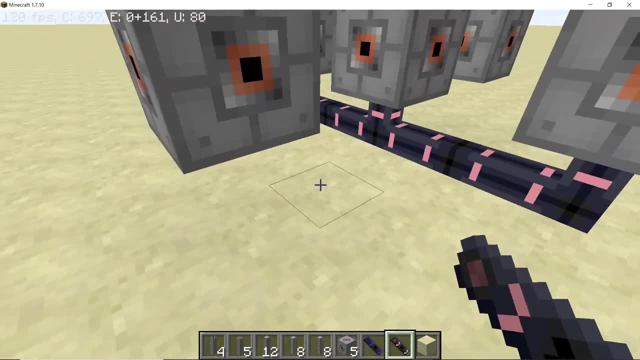 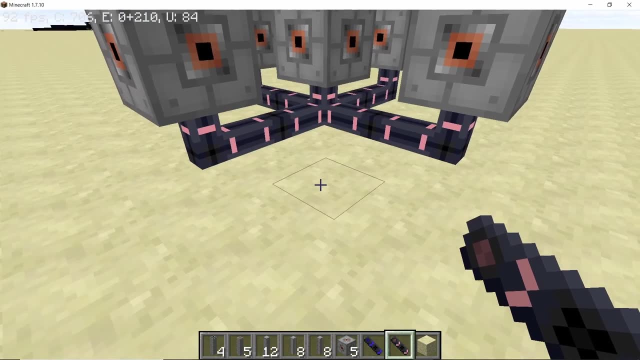 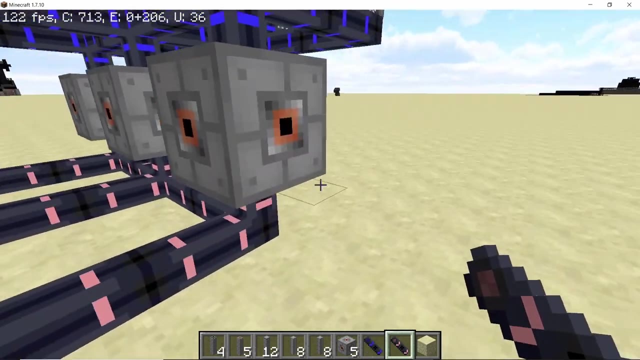 on the most lower block, place down your ultra dense steam pipes- as we are going to produce ultra dense steam using this reactor- and also connect them, like we connected the water ducts on the outermost block and put the second one into the outermost block, like this. 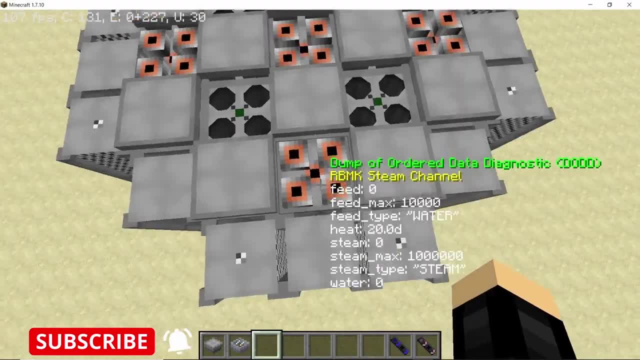 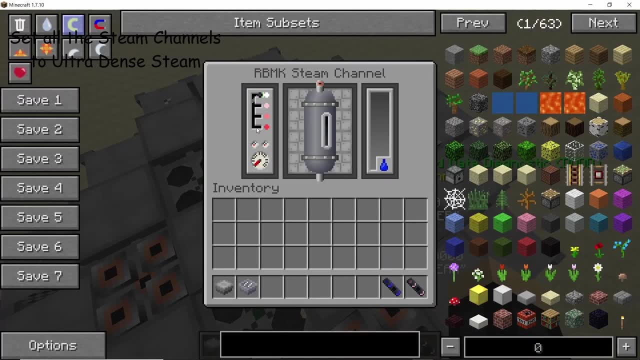 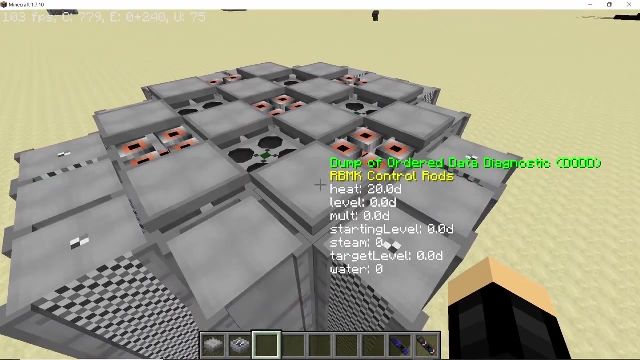 and finally the last one. there we go, with the piping done. now it's time to set all the rpmk steam channels to produce ultra dense steam. so here's the third rpmk steam channel. fourth and finally, the fifth one. now, also don't forget to set each. 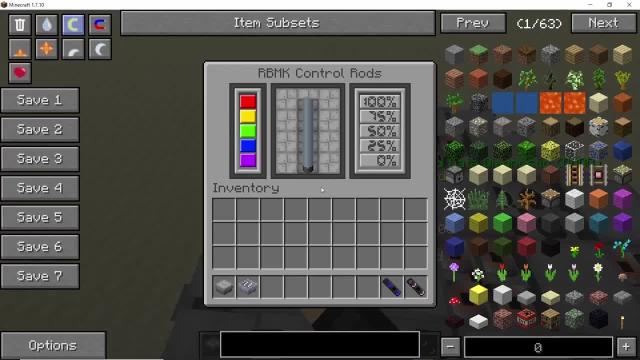 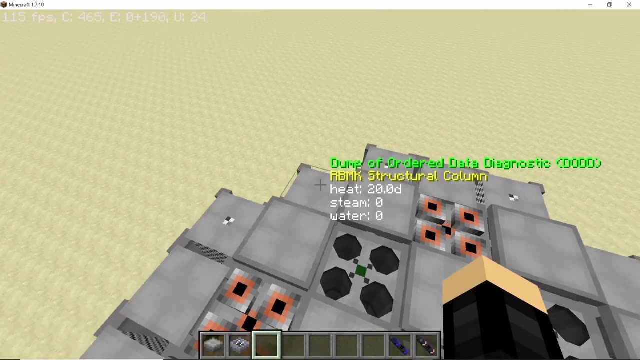 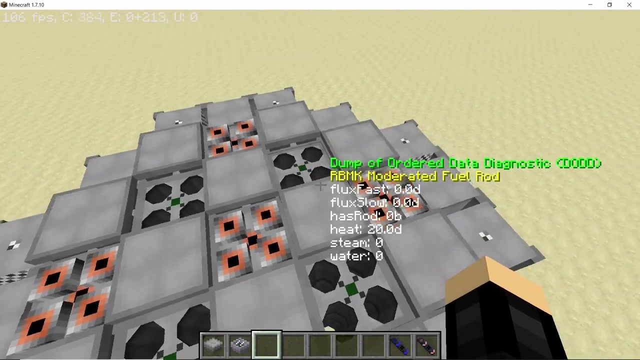 a specific color. i'm gonna go with red color here, but you can select any color you want. to just make sure that all the control rods are on the same color so that we can control all of them at the same time. and the last one now in order to double check that: whether we set all the control. 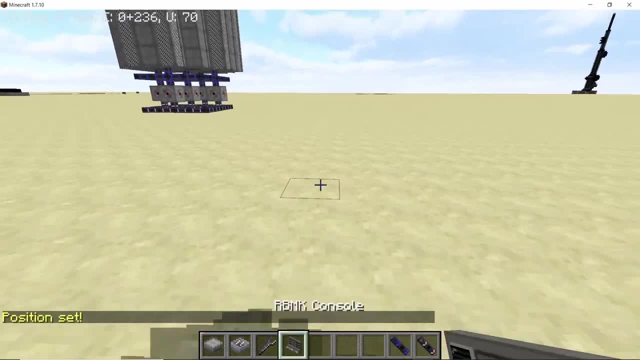 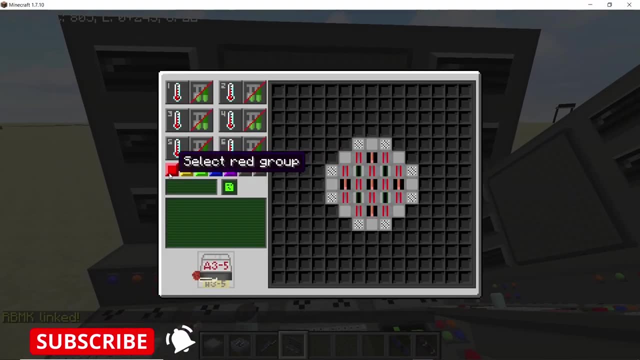 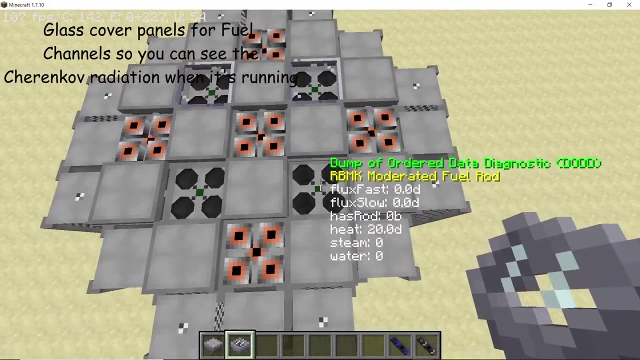 rods or not. i am going to link this rbmk with an rbmk console, so here it goes, and now when i go in this console and select this color red, it should select all the 12 control rods. so we have done that properly. now cover all the four fuel rods with the glass panel and all the other rods with the rbmk panel. 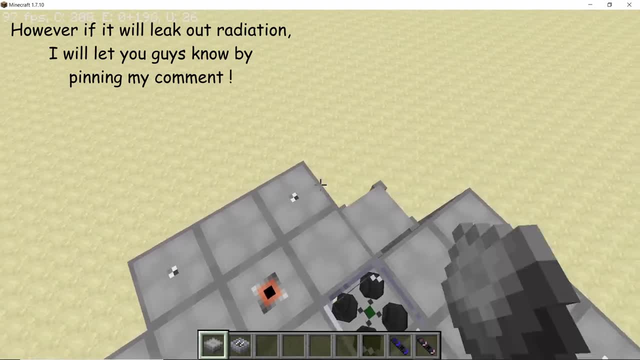 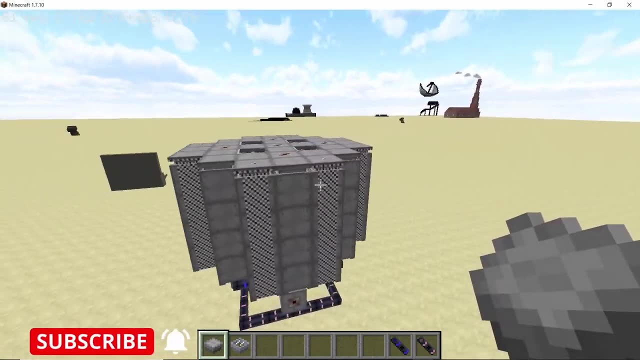 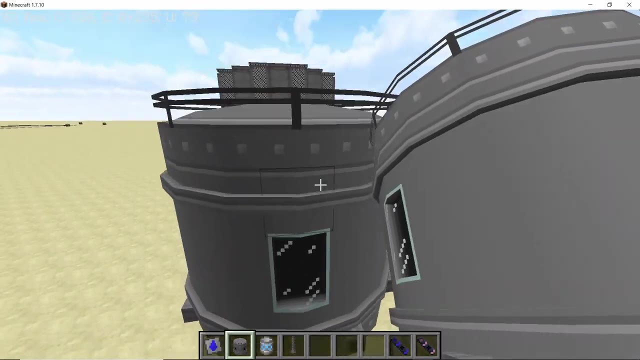 now you don't have to worry about radiation in this reactor, as it won't leak out, and i have tested it and, yeah, it will work perfectly without placing any radiation absorbers whatsoever. now it's time to set up the water supply, so place down a tank. i'm gonna use the biggest tank here. 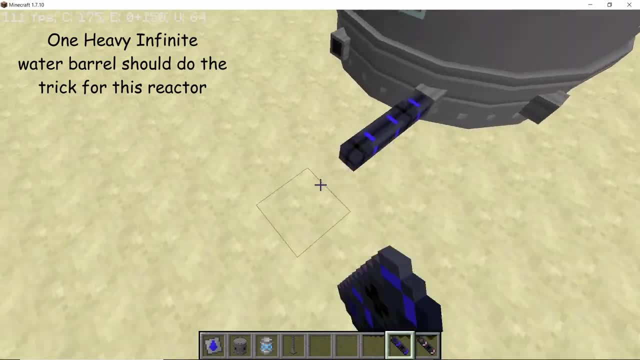 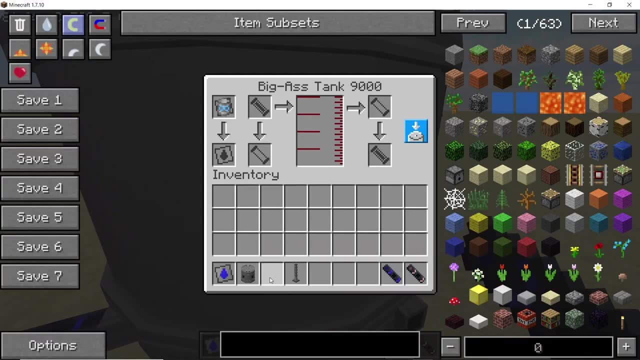 and place down an infinite water barrel in it and connect it like this with the rpmk reactor. so here goes the heavy infinite water tank, and make sure to set this water tank to input output now. as soon as you do that, all the steam channels in our rbmk reactor should fill up with water. 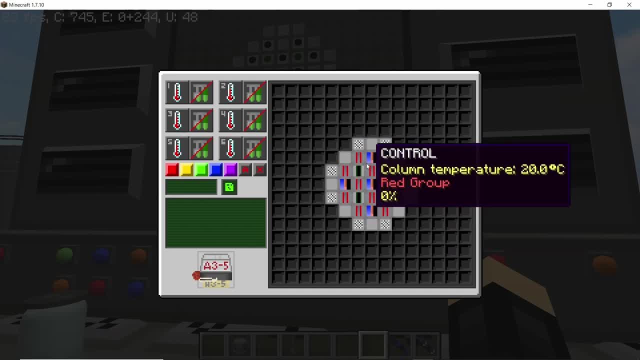 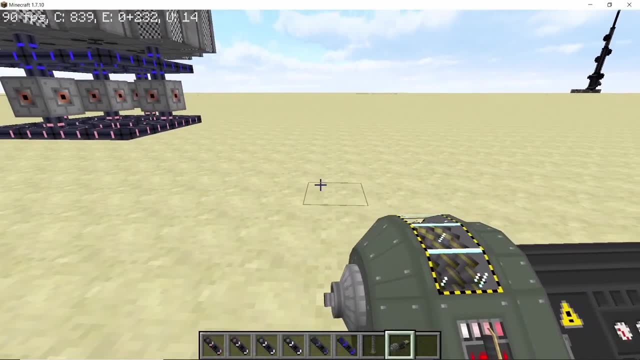 and we can see that using the console- rightly so, as you can see, all the steam channels have filled up with water. now let's take out the output steam, so place down four leviathan steam turbines. it's preferred that you use the leviathan so that there is no blockage of steam anywhere. 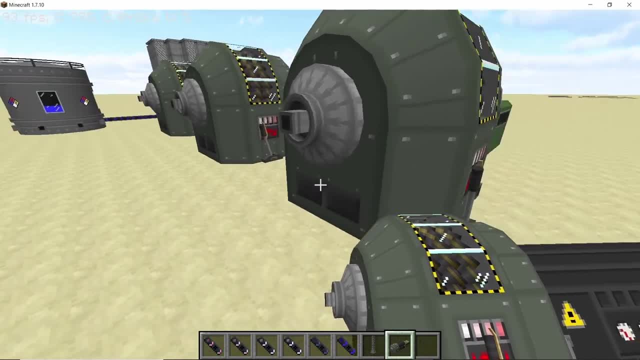 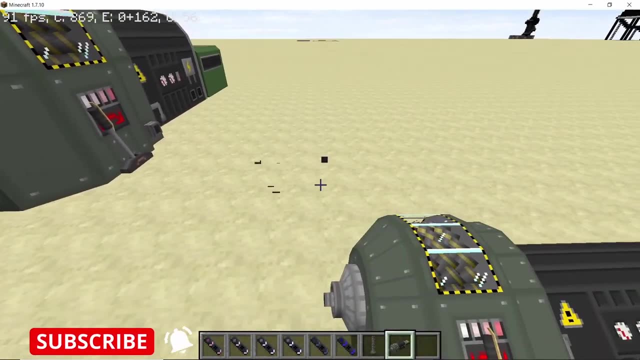 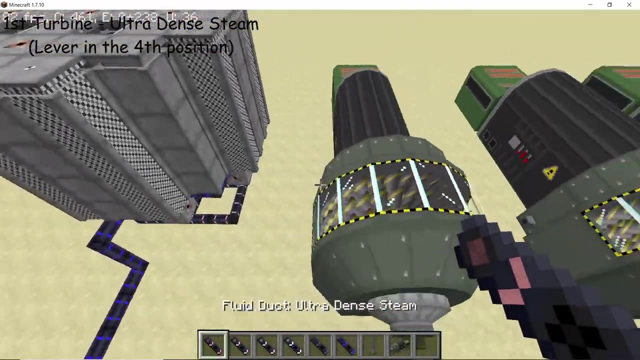 in the system. so three and finally the fourth one. you will need total of four turbines to do this. there we go here. okay, so the first steam turbine is gonna be processing ultra dense steam, so take out the ultra dense steam pipe and connect it to the first turbine like this, and also set it up to 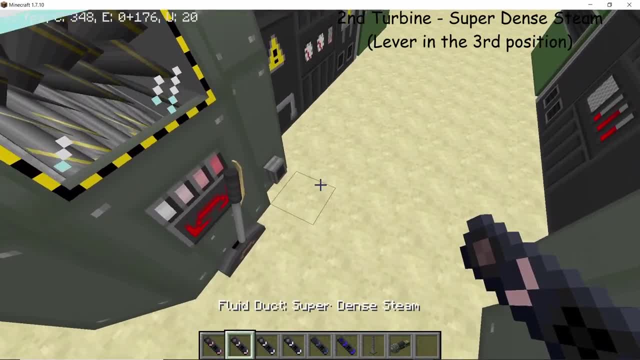 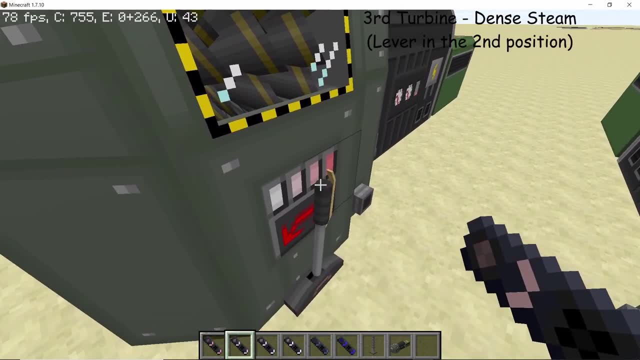 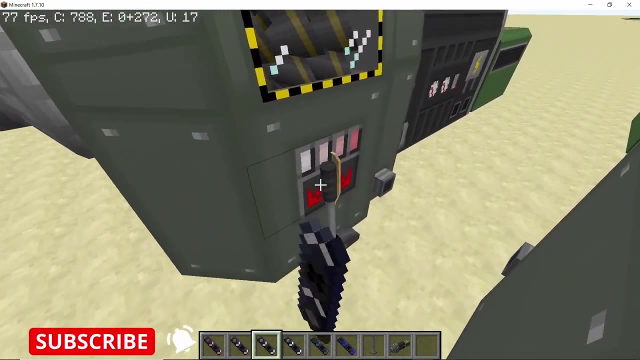 ultra density. now it will be converted to super dense steam. so take out super dense steam pipe second turbine and set this turbine to super dense steam like this, which will then be converted into dense steam. so the dense steam pipe goes into the third turbine like this: set it up and the dense 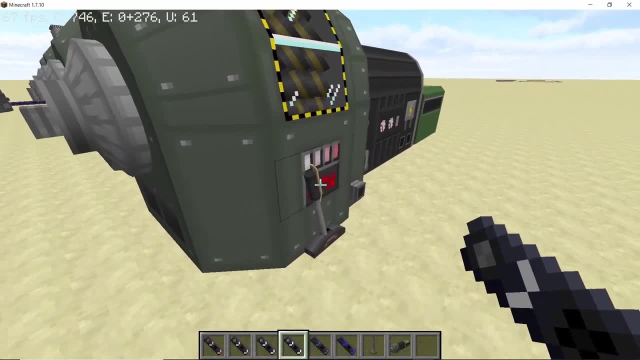 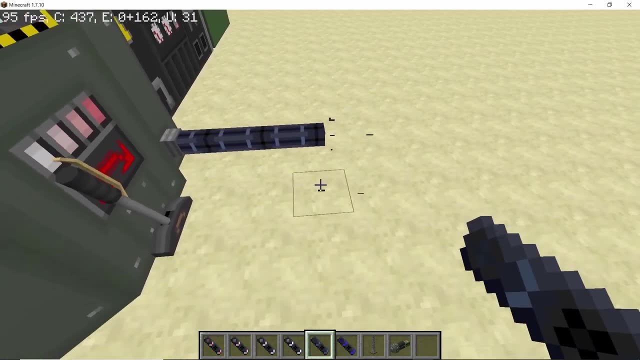 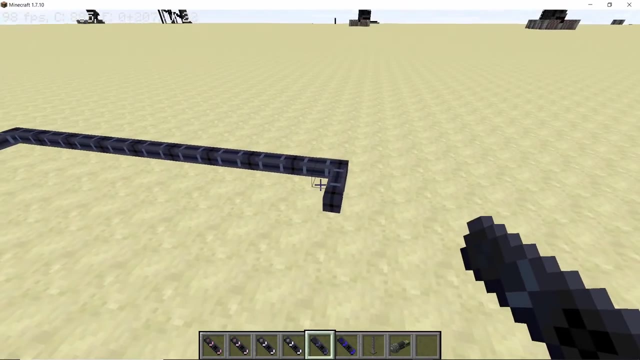 steam will be converted to normal steam, which is, by default, the default state of leviathan steam turbine. now take out your condensed steam pipe or low pressure steam pipe from the fourth turbine and bring it all the way back like this, because we will now connect this low pressure steam into our cooling tower, which will 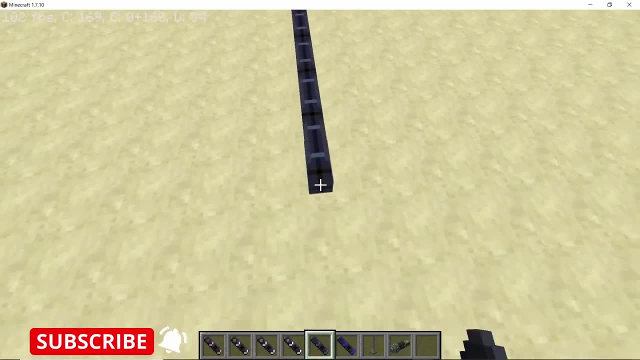 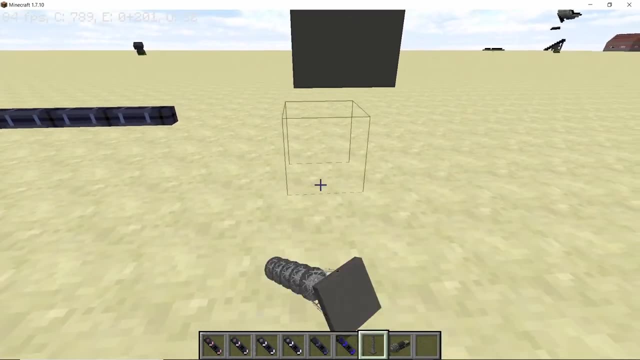 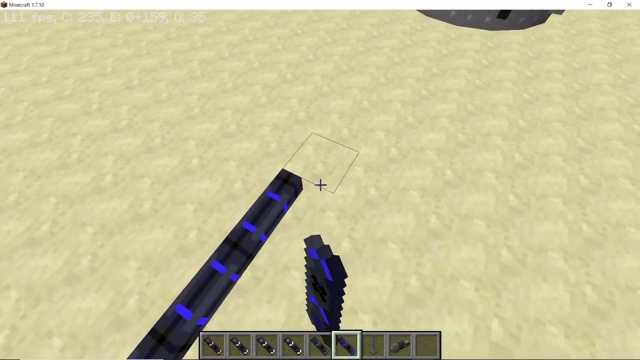 condense it into water, thus giving us a closed loop. so once we are nearly halfway there, place down your cooling tower- i'm going to use an auxiliary cooling tower here- you can use the big cooling tower if you want to- and from there bring out some water pipes going into our biggest. 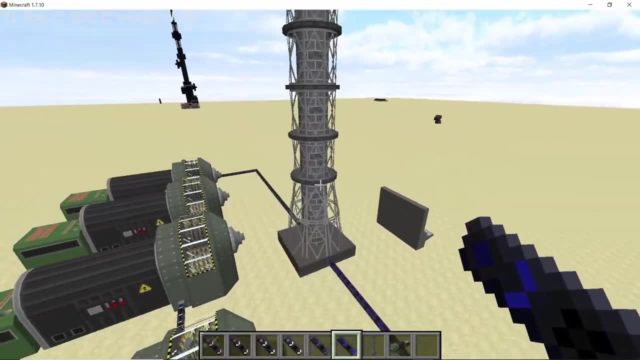 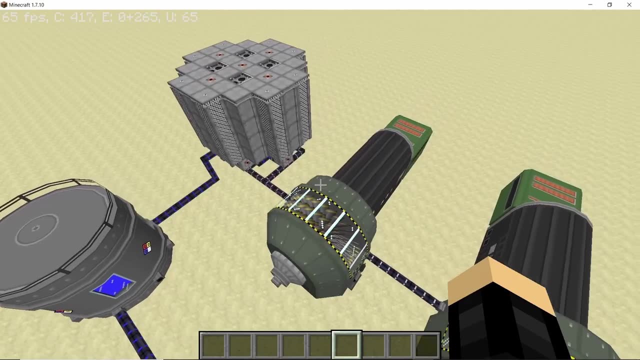 tank here and with this our loop is connected to the third turbine and we will now connect this low pressure steam pipe to the first turbine. so we will run the system. so this is the third turbine and this is our service tank now. we will now run the solution and then the system will. 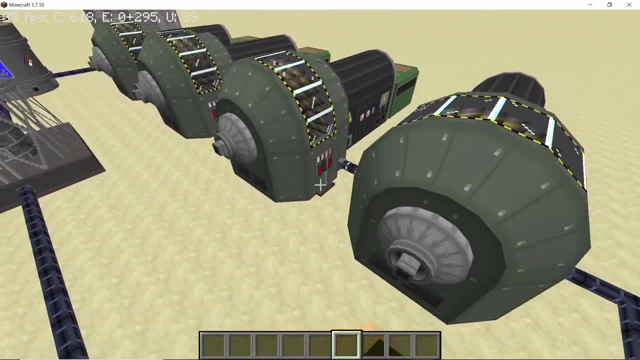 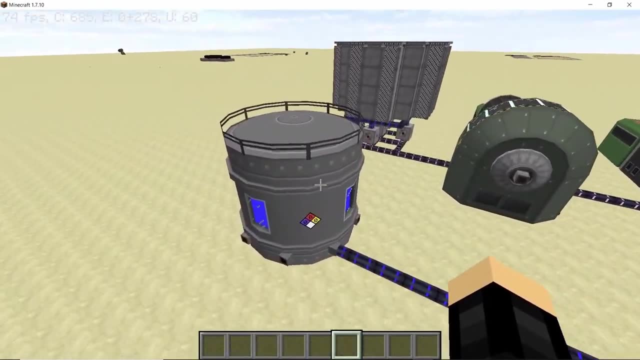 be complete once the loop is completed. so now we have completed our rbmk setup here and we are ready to run it. now. one thing that you need to remember is: this is ultra dense, this is super dense, this is dense and this is normal steam. don't mess this up, otherwise it will jam your entire system, and that is never good. 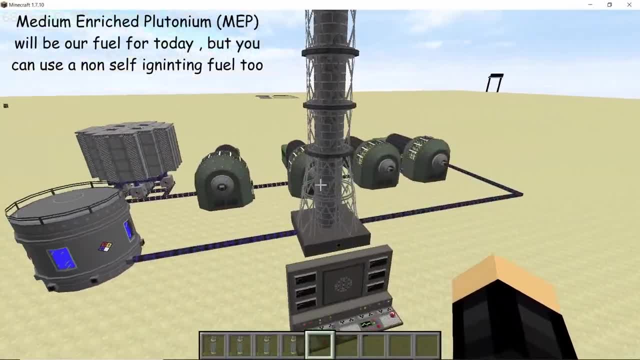 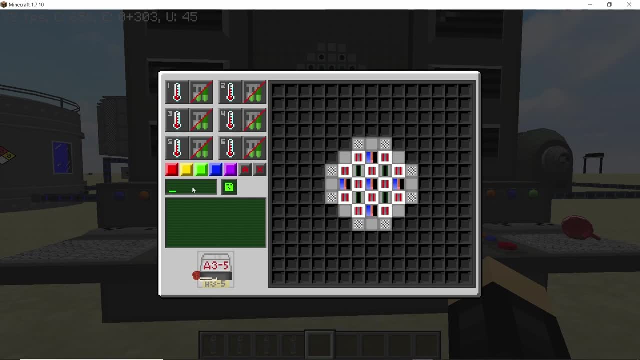 also here- make sure that this tank is set to input output mode. that is pretty important as well. now, in order to start producing power from the rbmk reactor, the very first thing you will need to do is pull out all the control rods by 20 percent, so select the red group type in 20 and 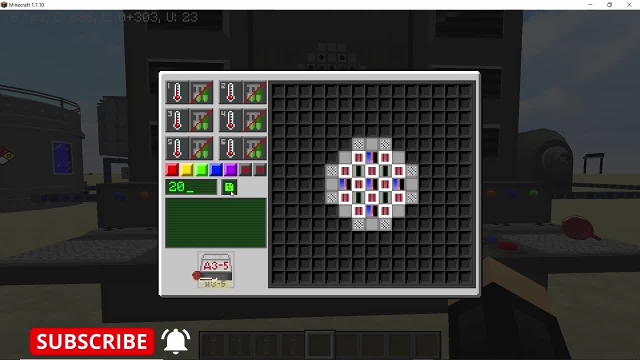 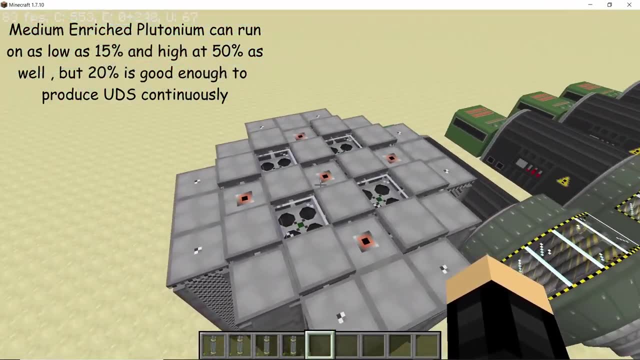 press on the save button and that should pull out all the control rods by 20 percent. now, when you are using medium and rich plutonium, you can even run this reactor at 50 percent, but it is best to run it at 20 percent, as 20 percent is an optimum value for producing ultra dense steam in this case. 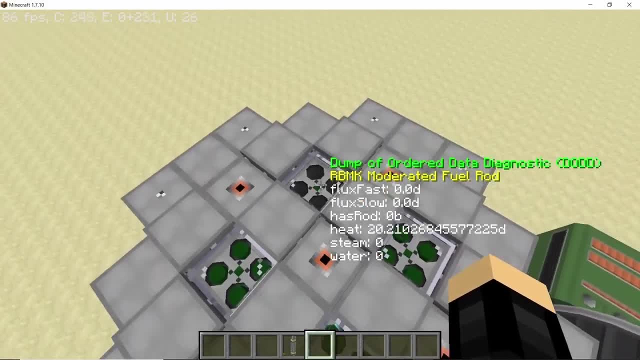 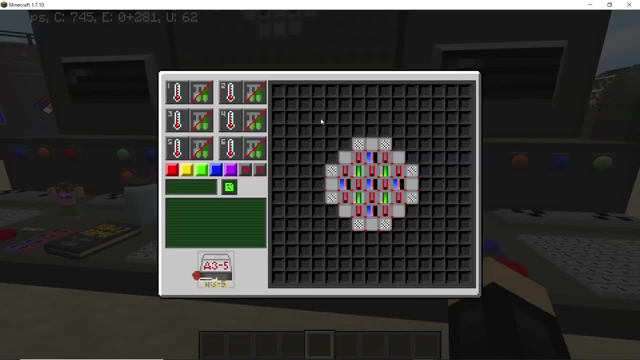 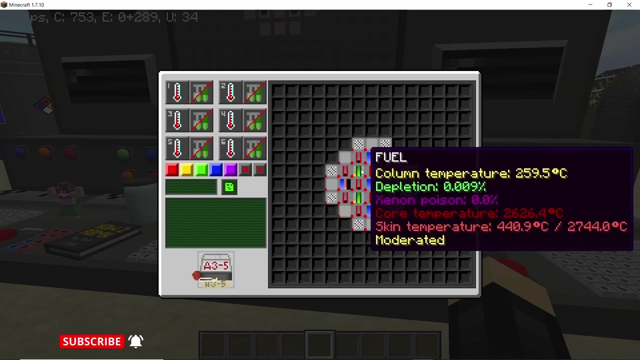 if you are using a different fuel, you will need to pull out the control rods in a different manner. but yeah, when we are pulling out the control rods by 20 percent, the skin temperature should go up to 855 degrees celsius when it has reached stability. so for now, you can see that the temperature is. 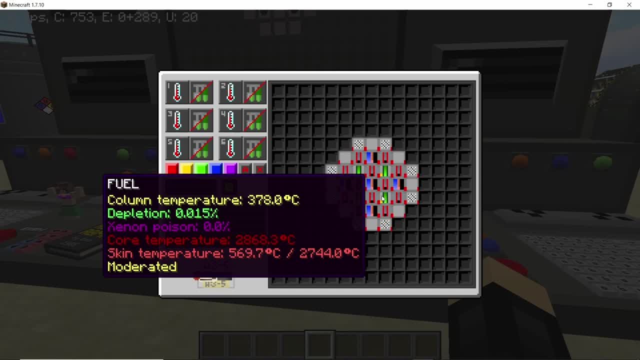 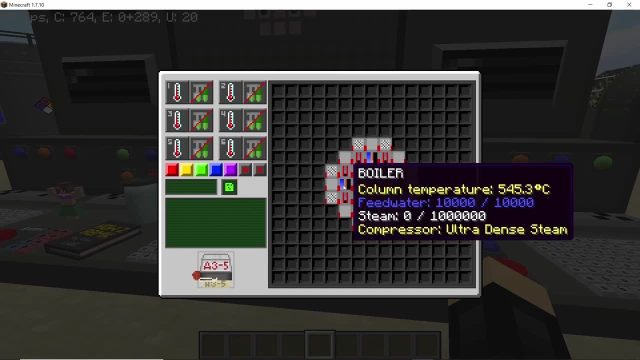 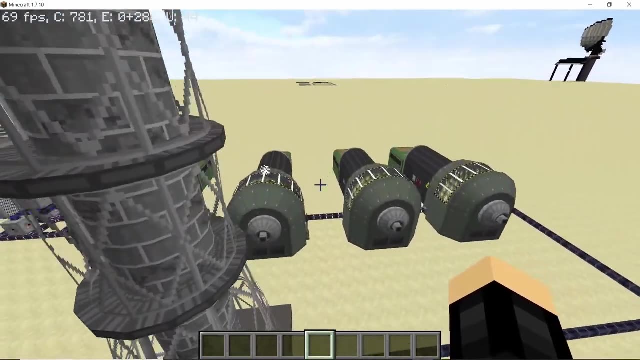 going up slowly, and as soon as this temperature reaches 600 degrees celsius, we will start producing ultra dense steam. so let's wait for it. it should happen really soon now. and there we go. so we have started producing ultra dense steam, and that means all our turbines. 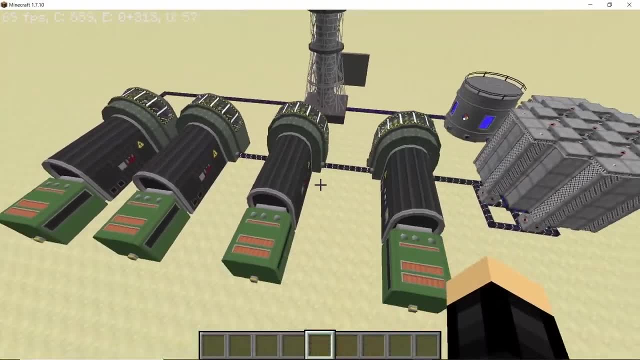 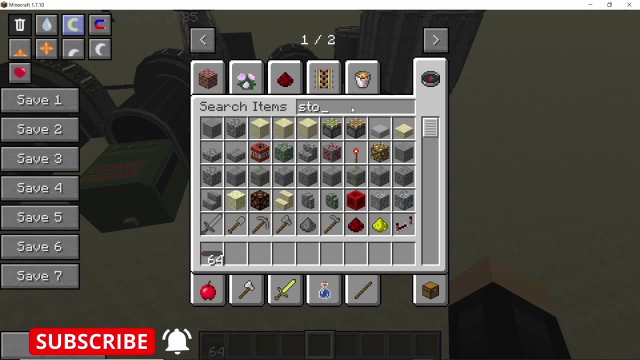 have started rotating. now, one thing that i forgot to do here was to actually take out the power from the turbines, so for that you will need some cables and some energy storage blocks. as i'm in creative, i'm gonna use the spark energy storage block, but you can use the lithium ion one, or yeah, basically. 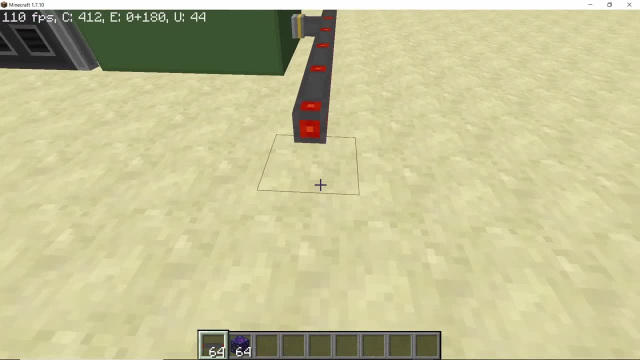 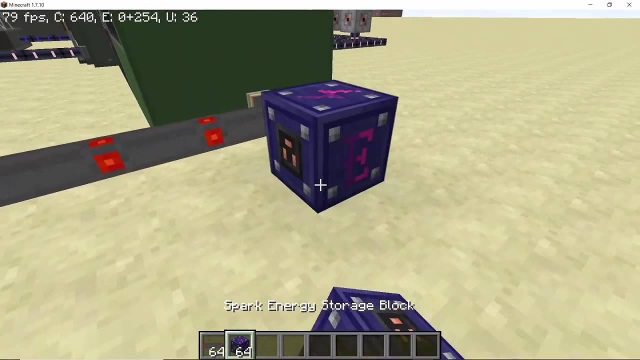 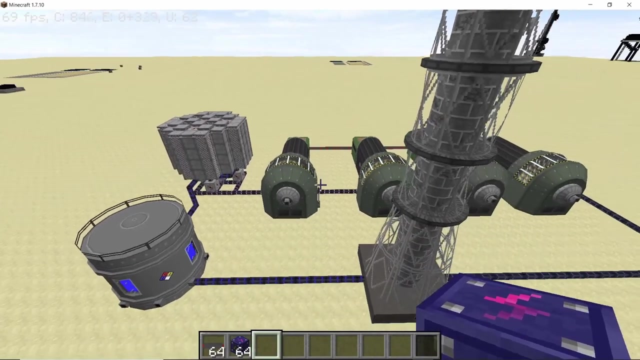 whatever you want to use. so connect all the turbines via cable, then just place down an energy storage block. so using the medium and rich plutonium as the fuel, it will give you around 3 million he per second. now that is quite a lot of power now, you do not? 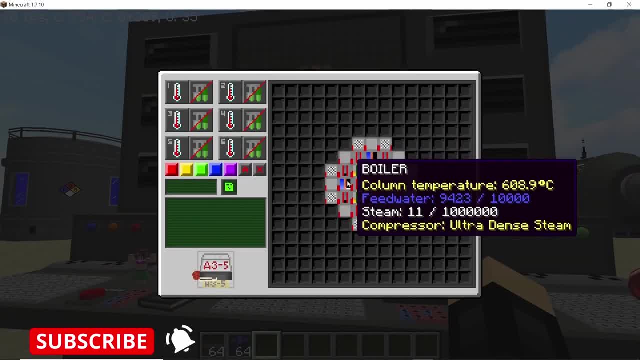 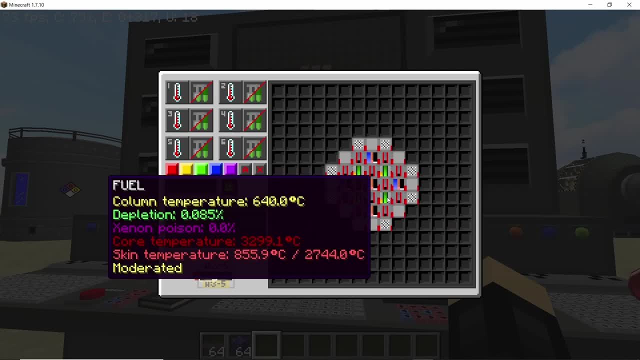 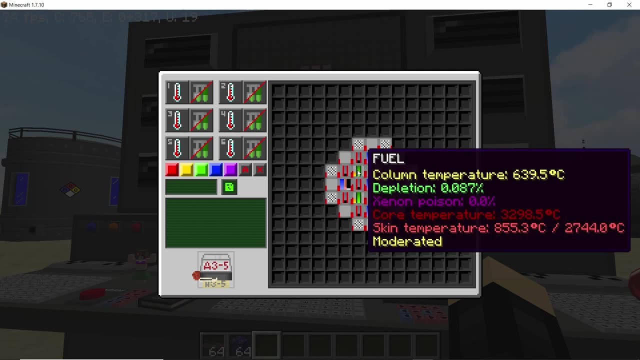 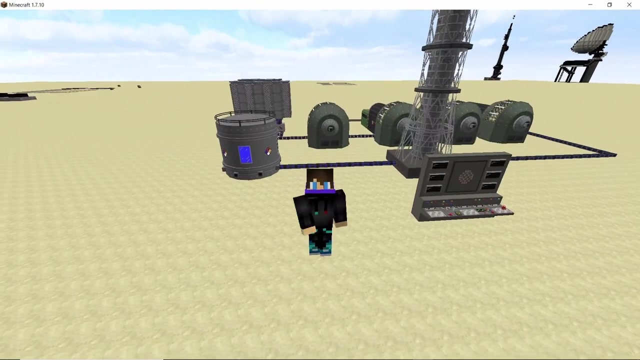 need to worry about this reactor exploding as, as you can see here, my reactor has achieved stability and all the all the rods, all the fuel rods, are at around 855 degrees centigrade. so, yeah, this reactor won't explode. at least in this update it won't, and yep. so this was the rbmk setup that i wanted to show you guys. it will run. 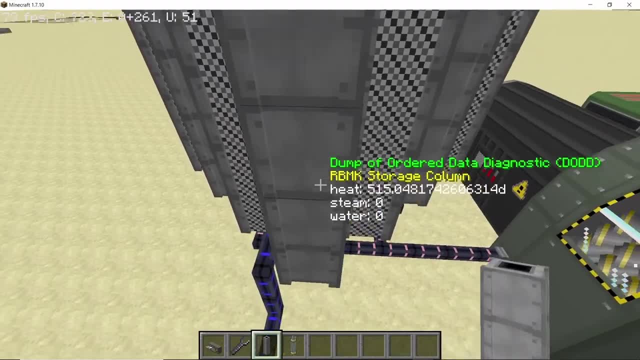 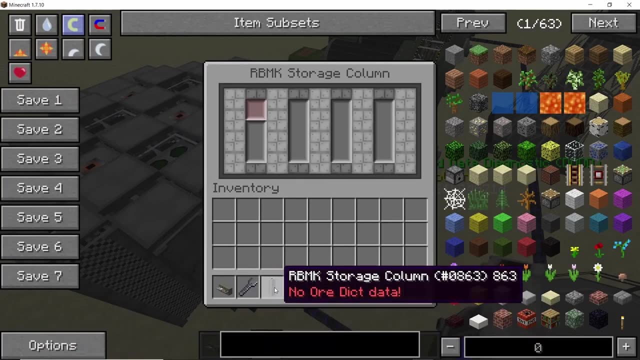 smoothly. and now let's see how to use the crane. so, in order to use the crane, you will need an rbmk storage column, a new block that was added. now, in this storage column we will place new medium and rich plutonium rods, so i'm gonna place six of them, and now we will link this. 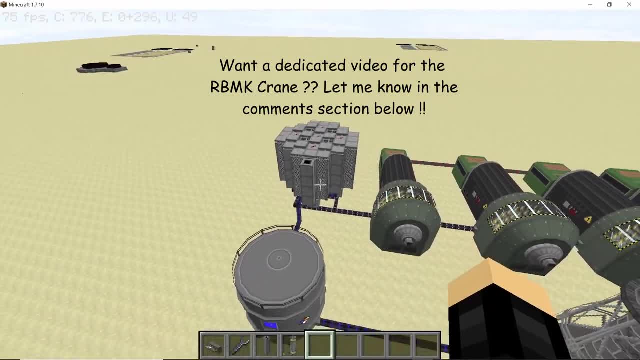 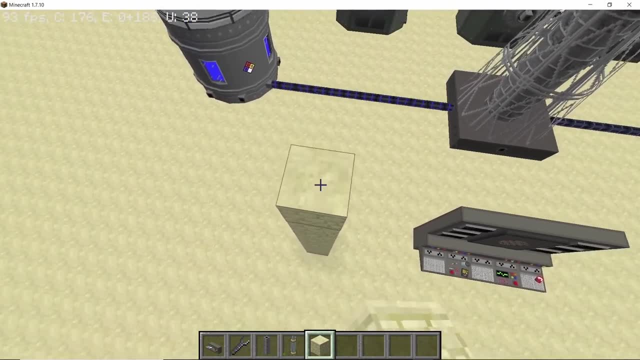 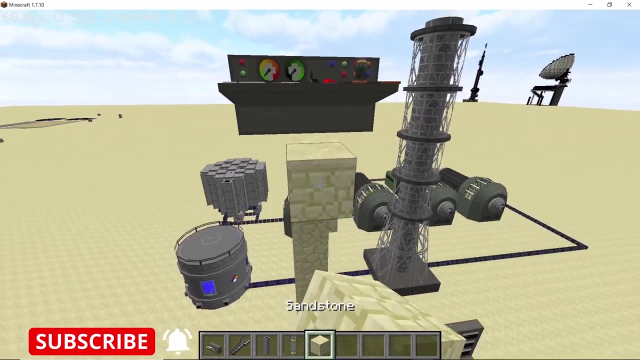 rbmk to the rbmk crane column or the crane console. sorry, not the column, but it is best to use this uh console at a height where you can see where the crane is going. so once i am at this comfortable height here, take the rbmk console linking device and 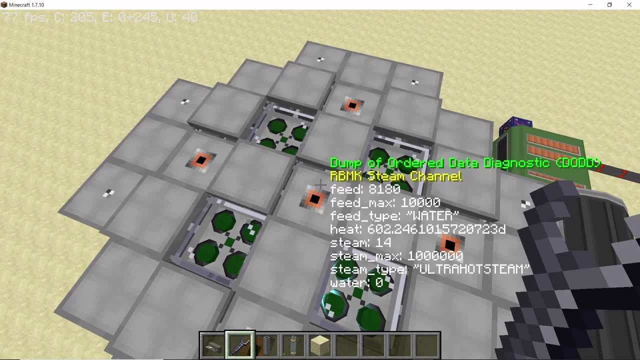 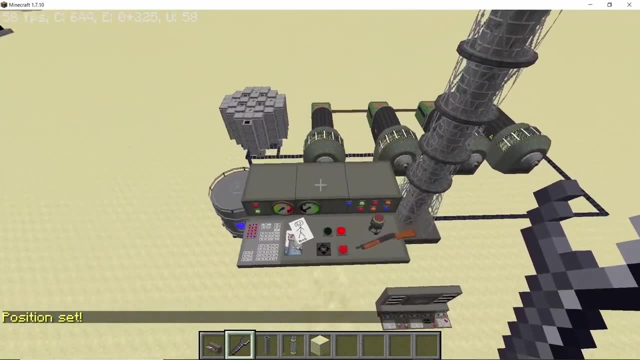 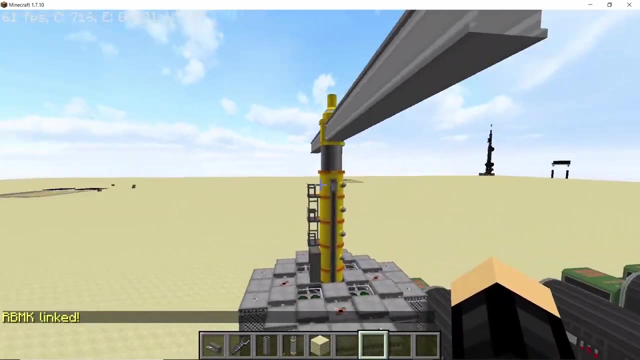 right click on the rbmk, basically the same step that you use in order to link the rbmk to the rbmk. so shift, right click on the rbmk and then right click on this crane console here, and as you do that, a crane will appear on top of the rbmk reactor. now, in order to start using this crane, 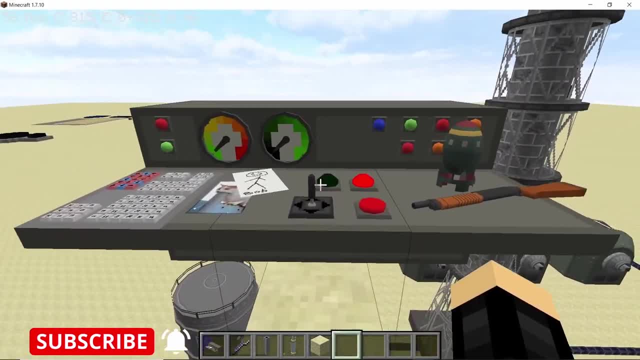 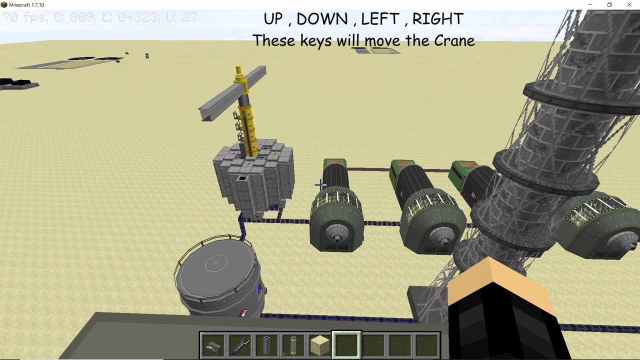 you need to stand on top of this console. yeah, you need to stand on top of it and then start pressing the arrow keys. so, using the four arrow keys, you can move the crane in four directions and in order to pull out any fuel rod, just press enter. so let's say that i want to pull out the fuel rod from this column right here. so i 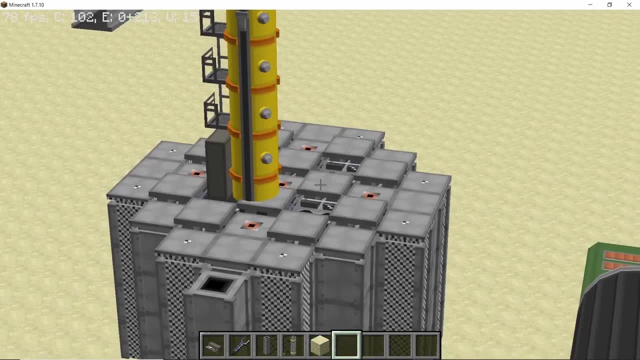 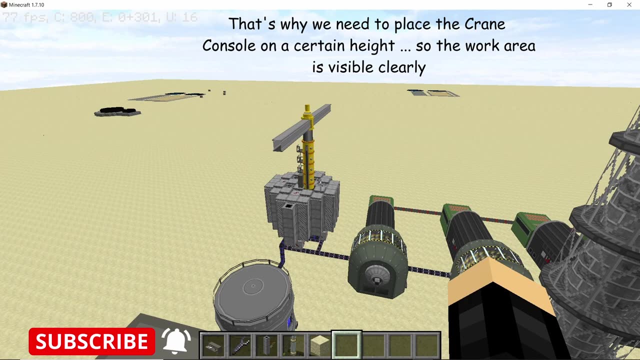 will press enter when my crane is on top of it. so this is the fuel rod that we want to pull up. so bring your crane on top of it and just press enter, and there we go. the crane has pulled out the fuel rod from that section here.